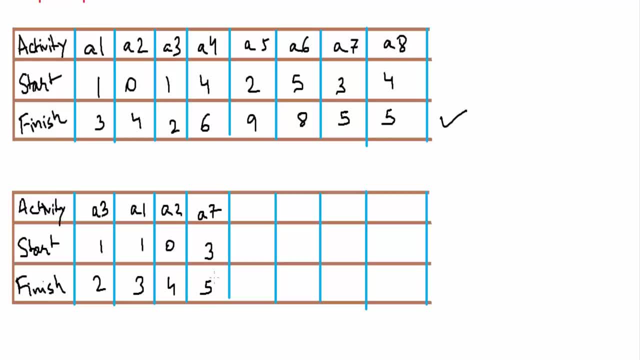 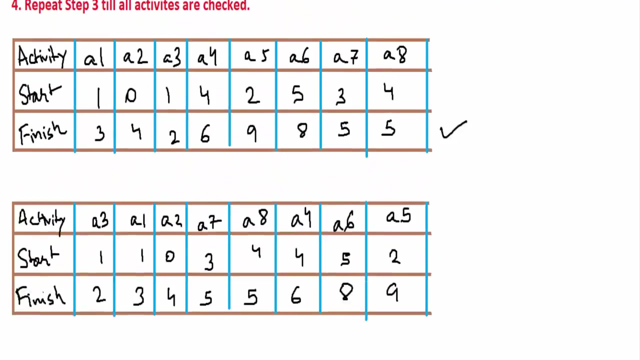 first, So its preference will be higher. So three, five, a eight, four and five, Then a four. This will be four, six, eight, six, five, eight. This will be a five, This will be two, nine. So now, since we have sorted the activities, so now we'll just select the first activity. So 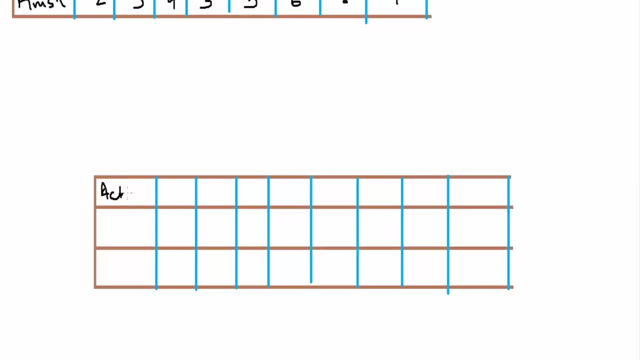 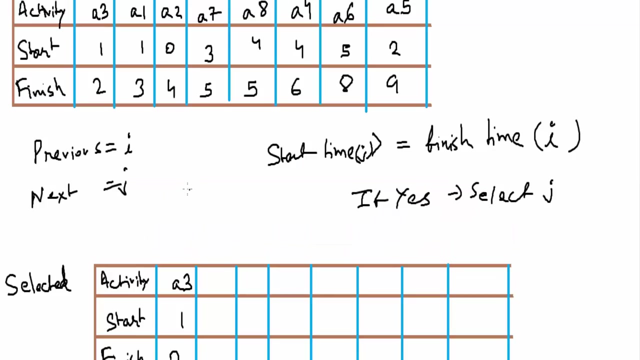 here we'll write the selected activity. So this is our selected activity. So this is a final chart or table. So again, we'll write the starting and finishing time. So we'll select the first activity. Our first activity was a three and its starting time was one and its finishing time was two. So here we see that, like our starting time is now what for a one, it is one and our 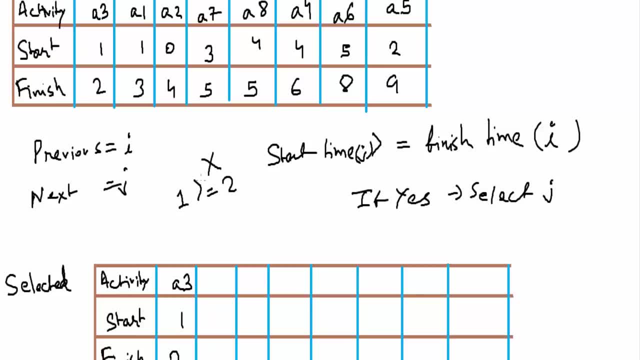 previously finished time was two. So this is not true. So a one will be skipped Now for, similarly for a two. So its starting time is zero, which is not greater than equals to two. So it will also be skipped Now when we come to a seven. So we see that, like, three is greater than equals to two, So it is- if, yes, it is selected, So a seven. This will be. 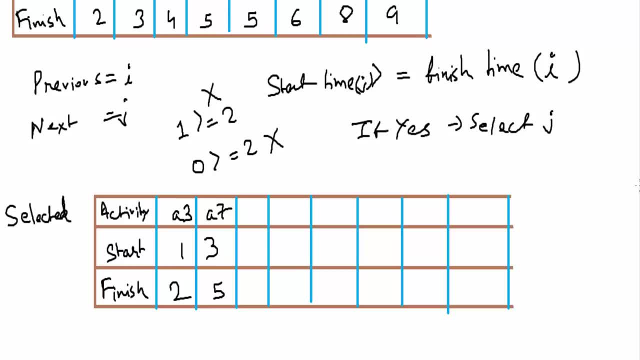 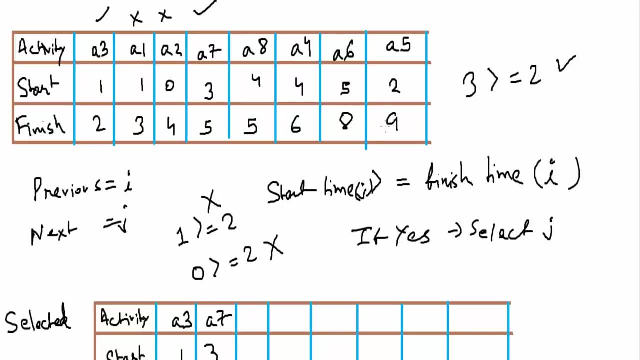 Pa three and five. Now let us see again. So now we have checked: a seven- This has been selected, This not. This is not, This Hasn't Selected Now. or a eight. So our starting time is what four for is not greater than equals to five, So won't be. 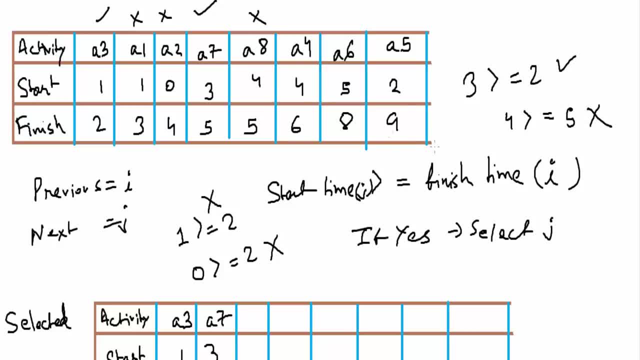 selected. So not again, not for a four. So four is again known. Brig어지 equals to five. So it is now for 5. so for 5 it is greater than equals to 5. so for a6, 5 was the starting time and